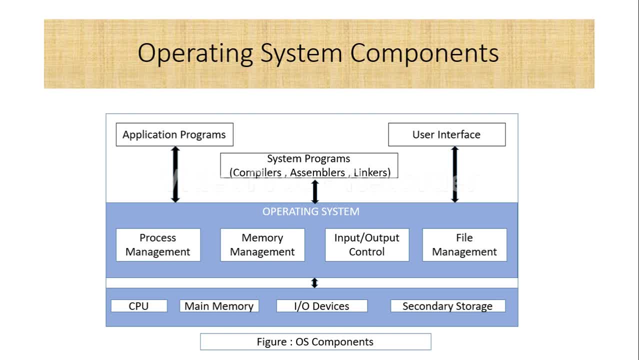 and this process management is also responsible for resuming of the process or suspending them. okay, so this kind of resuming and suspending will occur whenever the process requires certain resources to be utilized. it is also responsible for process synchronization, as well as communication also. and then, finally, the process management is also responsible for. 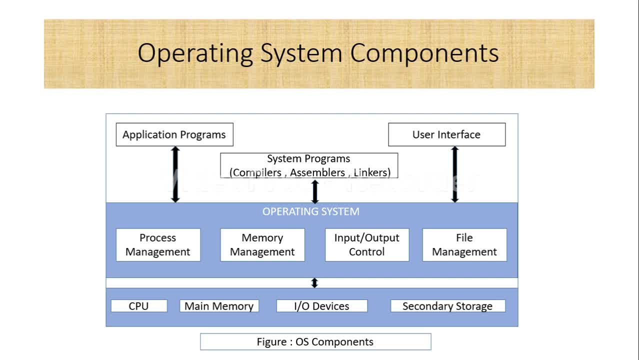 handling the deadlocks. okay, so process management is going to provide the techniques for handling the deadlocks. so this is about the process management overall. we can say: the process management is going to manage the entire process or the entire program which is in execution. then the next component is memory. 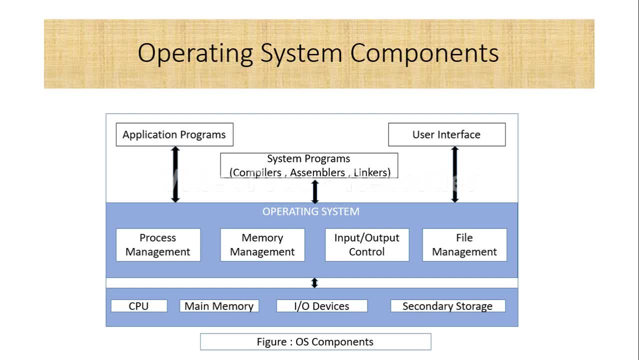 management. so, as we know, memory management is very important for the operations of the computer. okay, so basically it is the storage device which is accessed by the cpu directly. so if you see the memory management as a component in the operating system, so it is basically keeping track of the 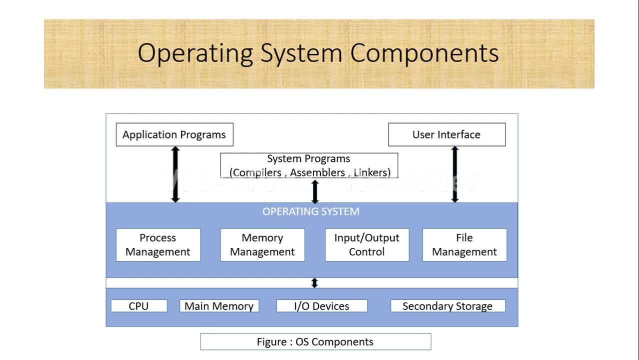 memory usage. that means it will keep track where exactly the memory is being used and who exactly is using it. when we say who, it is, basically which process is utilizing the memory. it is also responsible for selecting the process which should be loaded into the main memory and it is also responsible for 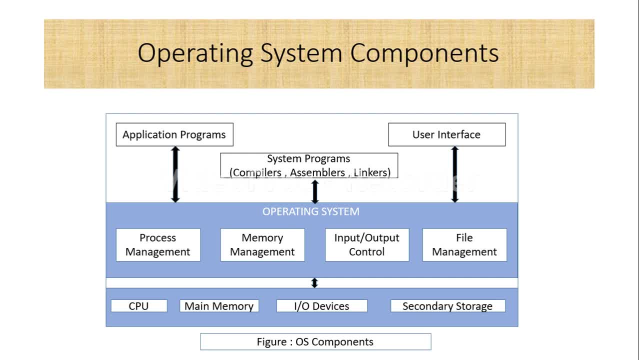 for allocation and deallocation of the memory when the process is executed or when the process is completed. it is also responsible for releasing the memory. okay, then the third one comes in the form of file management. as the name indicates, it is basically dealing with the management of the files. as we know, file is a collection of related information, and whenever we talk, 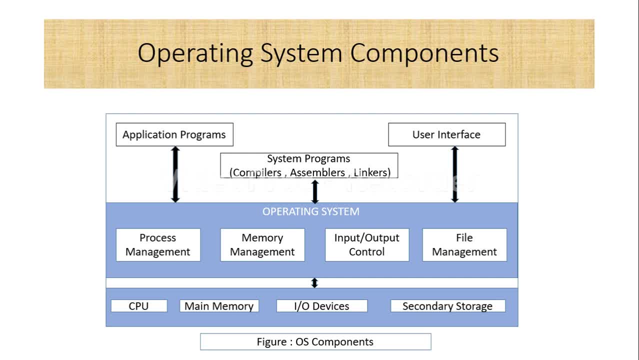 about this file management in the operating system. it is basically dealing with the creation of the file, deletion of the file and manipulation of the files. also, it is also responsible for mapping the files onto the secondary storage as well as it is providing backup for the In case, if it I mean due to certain reason- if your data is lost or if your file is lost, the file management is responsible for recovering the files and provide the proper backup. okay. 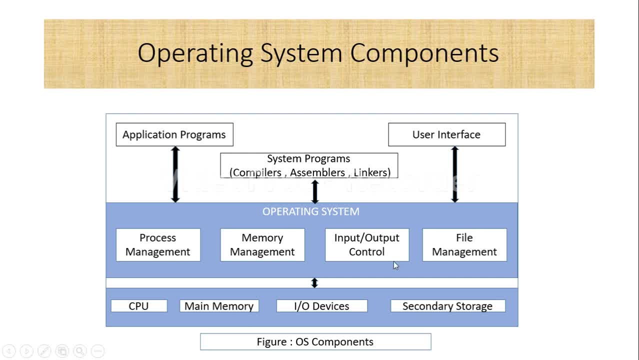 Then the next one is the input-output device management. This input-output device management is basically dealing with all the input-output devices. okay, Already we know what are the different input devices and what are the output devices. Now, the main purpose of using this kind of IO device management is to basically to manage the device drivers, to manage the input-output operations of the various devices, and it is also managing the memory components. okay. 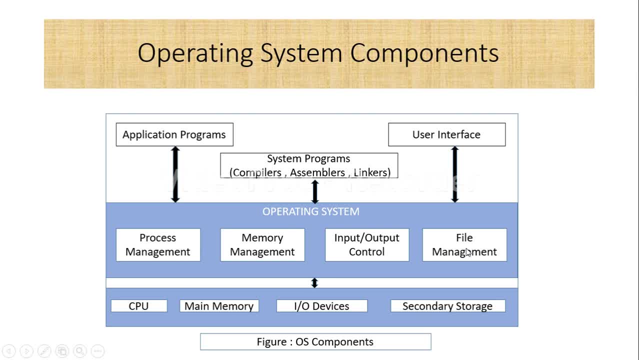 Then the next one. The next one is the disk management, or we call it as secondary storage management. okay, So here, basically, we are focusing on the management of the secondary storage, which we also call as disk storage. okay, So here, basically, we are focusing on the storage allocation, how exactly we are scheduling the disk and how we are allocating the free spaces to the different processors. 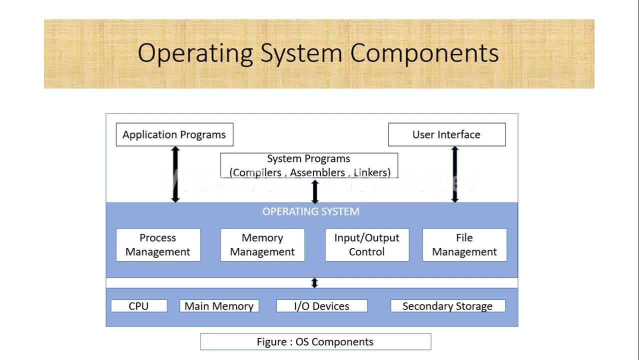 Okay, then we are having the next component, called as networking. So networking is nothing but where we are collecting the programs and we are going to. I mean, there is a process of communication with the various processors, and this communication is happening through the high-speed buses. okay, 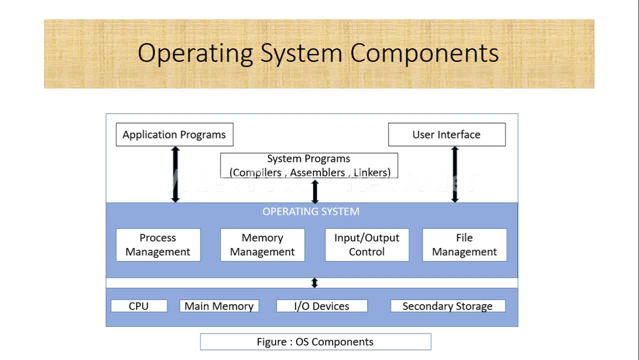 So whatever the set of computers are there, they are basically interconnected with the hardware, So there is a type of communication network. Then also we are having another component called protection system. This protection system is basically controlling the access of the program, or how the user is able to use the resources. okay,